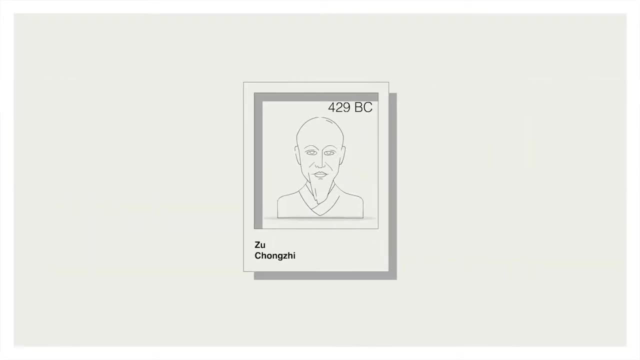 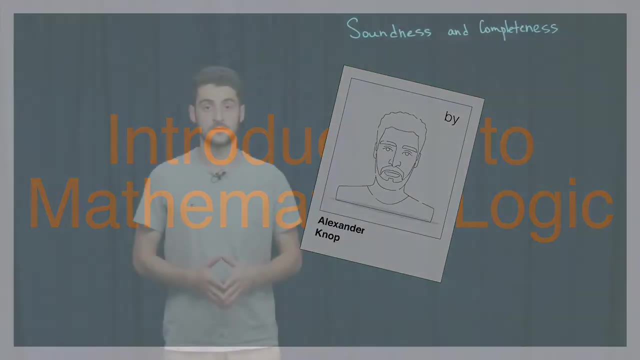 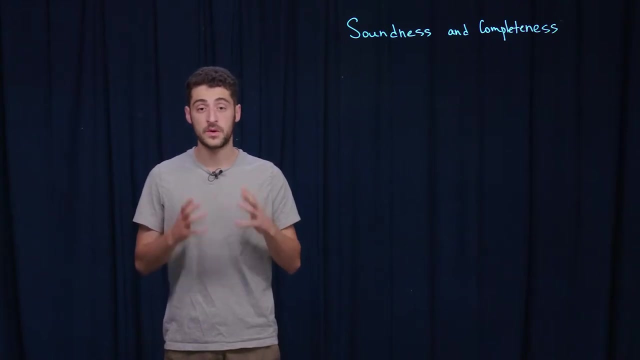 Hi, my name is Alexander Knop and this is Introduction to Mathematical Logic. In the previous video we defined natural deduction. In this video, we are going to discuss two of the most important properties of this system. They are called soundness and completeness And soundness. 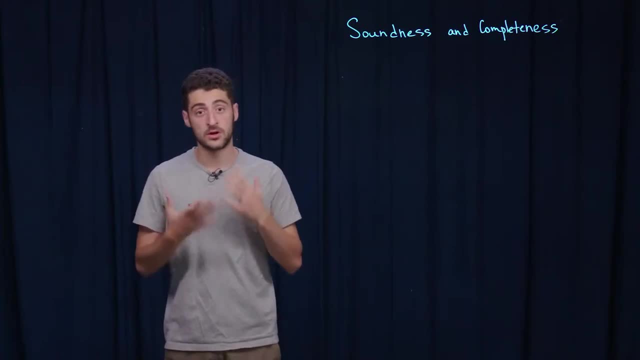 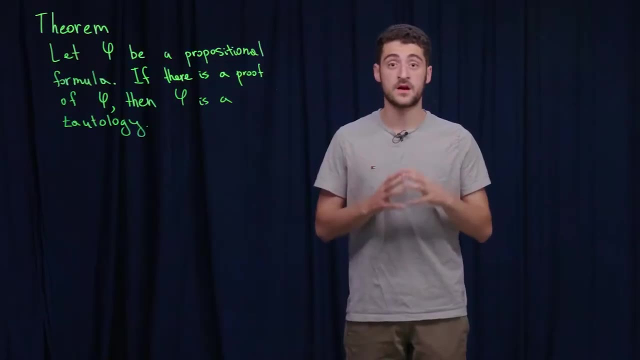 says that if you can prove something, it's a tautology. Completeness, on the other hand, says that if you have a tautology, you can prove it. Let's start from the soundness. Formally, the soundness property is the following: If you have a formula phi, a propositional, 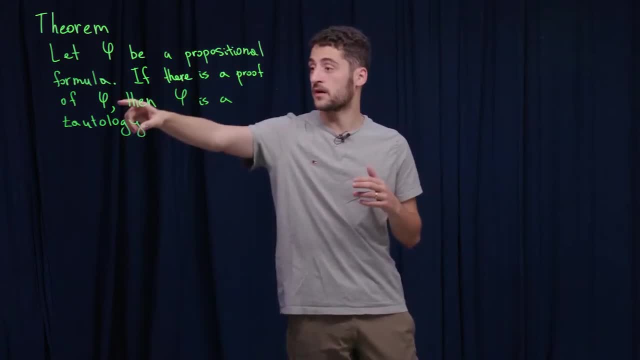 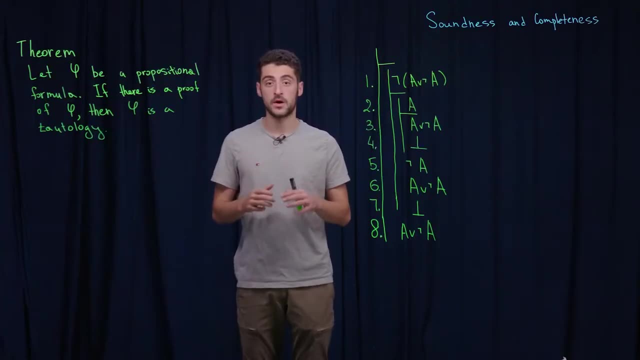 formula, then if there is a proof of phi, then phi is a tautology. The proof of the theorem is a bit too technical for this video, so we are going to illustrate it with an example, with the hope that it's easy to follow. So the example we are going to use is the law. 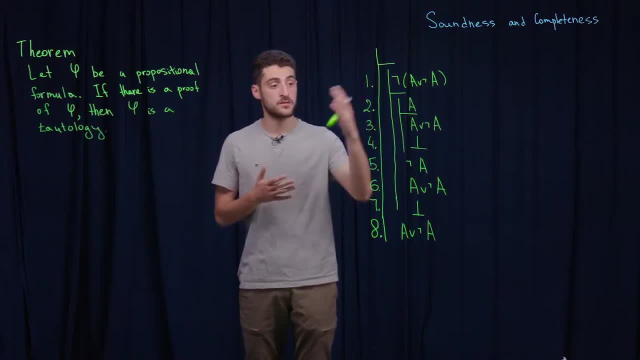 of excluded middle we proved in the previous video. The proof was like this. So what we are going to do is the following: We are going to replace every line of the proof by a propositional formula, such that all of them are tautologies, and we'll finish with the tautology we wish. 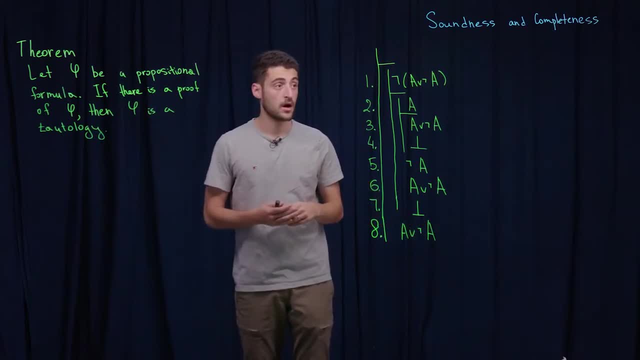 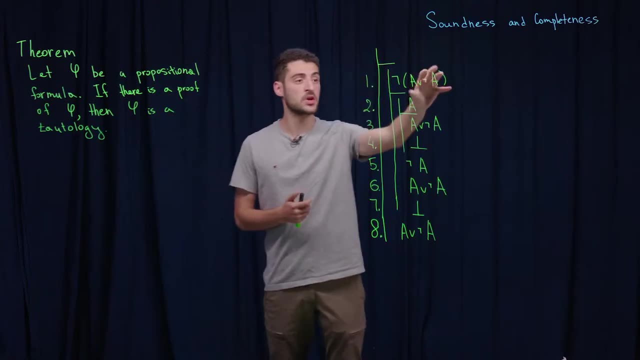 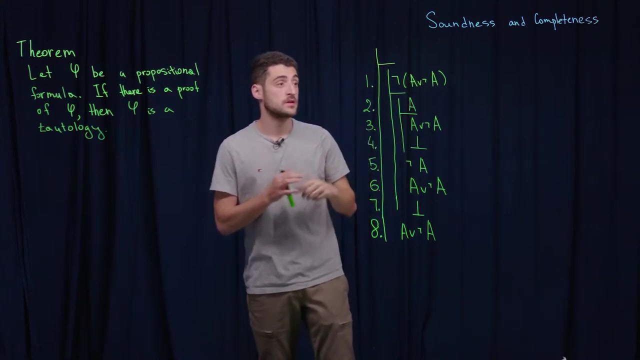 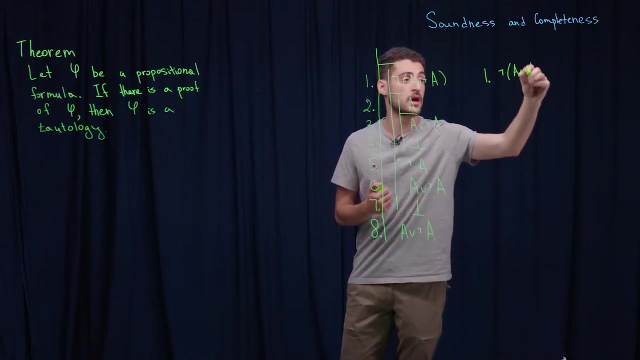 to prove and it will prove the theorem. So we start with an empty line because we don't have any assumptions, and the first actual line is an assumption that a or not a is not true. We rewrite it like this: So we say that under the assumption that a or not a is not true, we can derive the assumption. 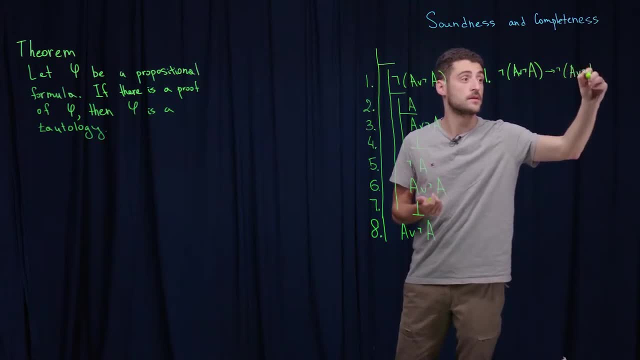 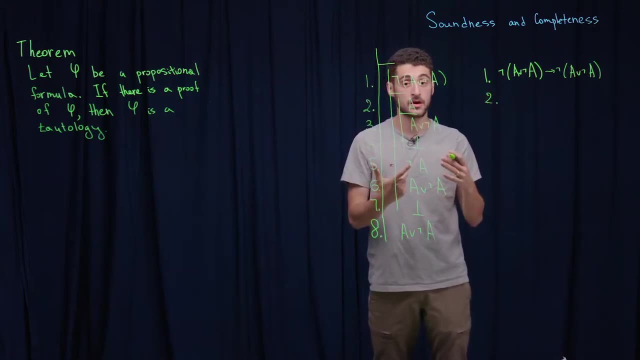 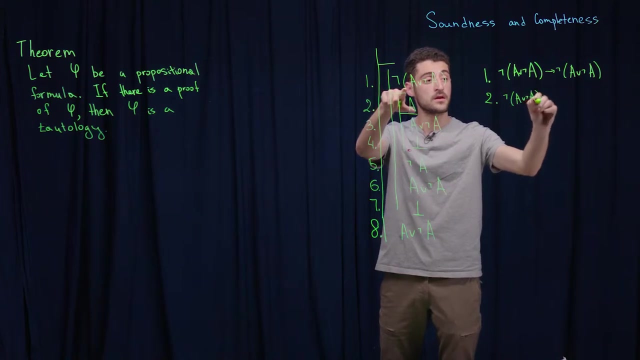 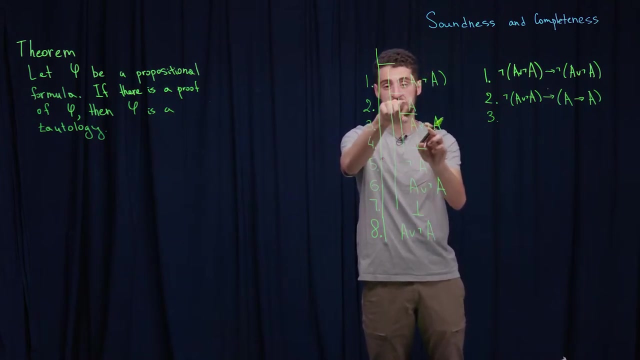 itself. The next step is creating a new assumption. So we say that under the assumption not a or not a assumption, a implies itself. Finally, we have the third step, and the third step is introduction of disjunction from the second step. 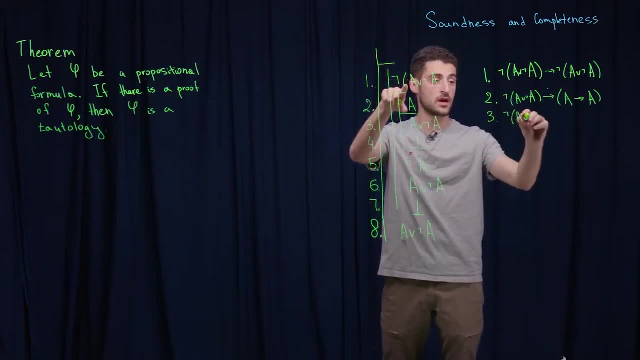 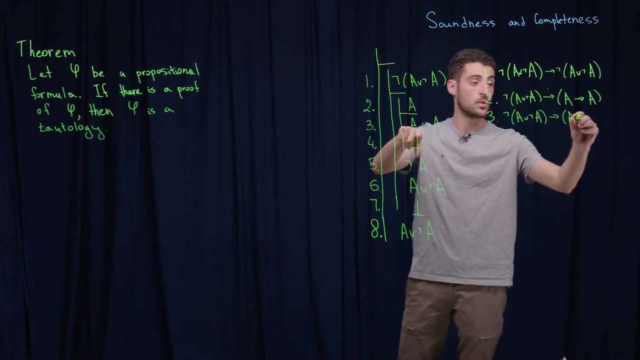 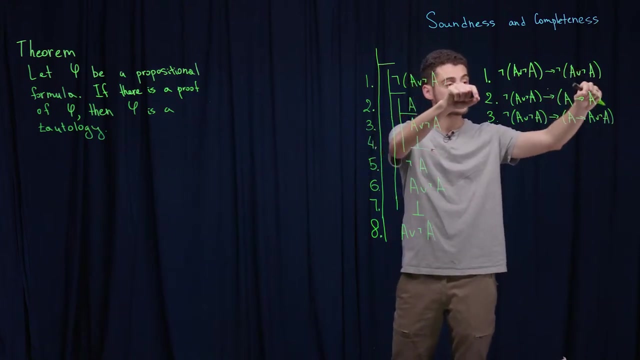 It's under the assumption that a or not a is not true And assumption a: we know that a or not a should be true. Note that these two formulas are tautologies just because the assumption and the conclusion are the same Here. we knew the fact that this is a. 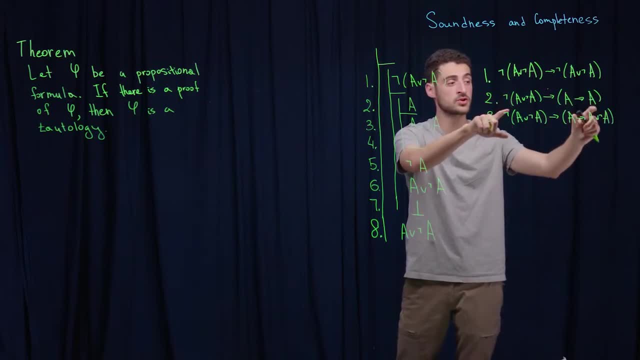 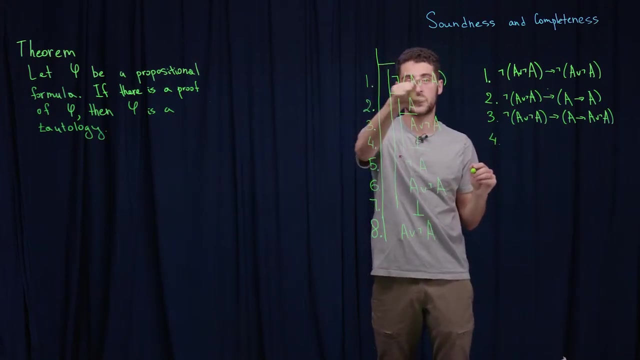 tautology and we replace by the conclusion that the conclusion is true or something else, And in other words, this is still a tautology. After that we have the first step. we concluded that, under the assumption that A or not, A is false and A is true, we 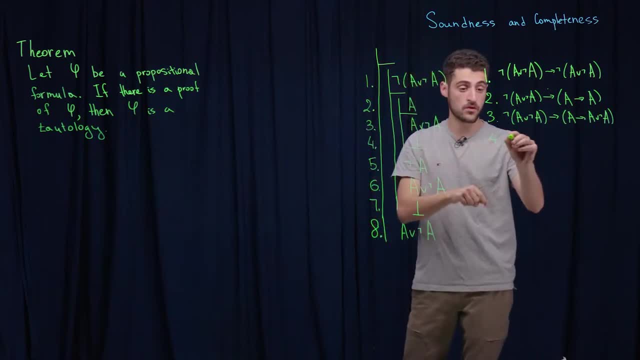 get a contradiction And we rewrite it like this: under the assumption A or not, A is not true and under the assumption A, we get a contradiction. Now that this is also a tautology, because the third one was a tautology. You had an. 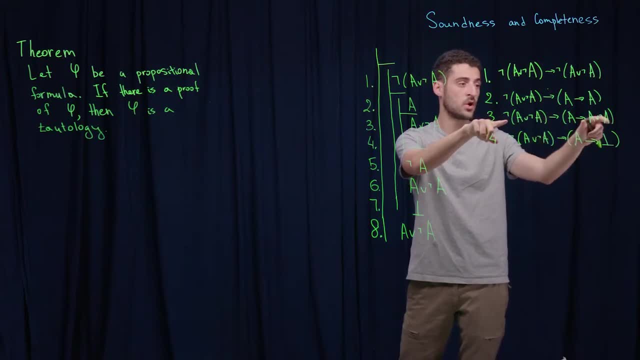 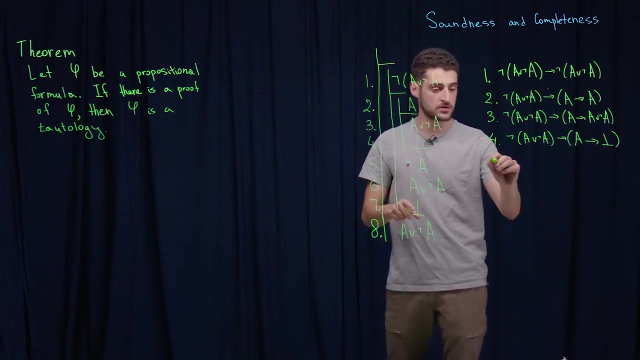 assumption that A or not A is false and you got a conclusion that A or not A. In other words, it's a contradiction, because they cannot be correct at the same time. so we get a contradiction. Now we got rid of A and we derive a conclusion from it. We stretch them to the相. Thank you. 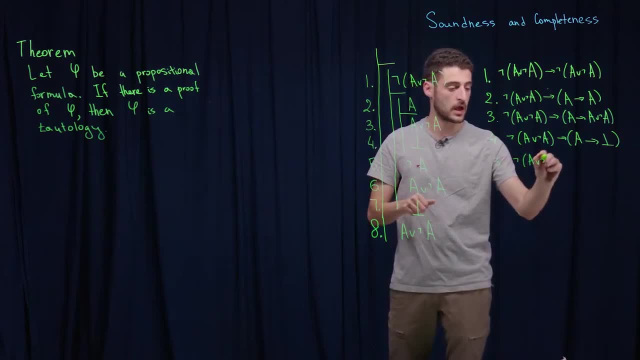 that, under the assumption that A or not A is not true, we get not A. Now that this is a tautology. because this is a tautology? because we, here, we have a conclusion that A implies a contradiction. In other words, not A is. 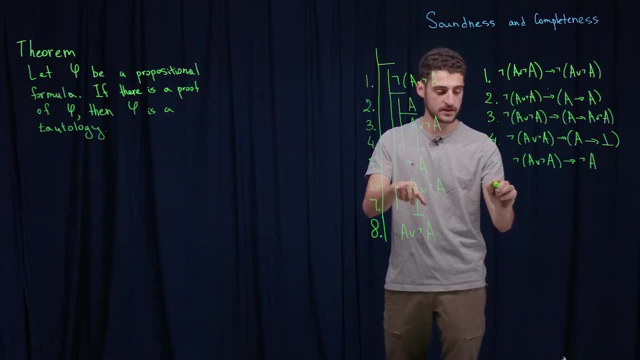 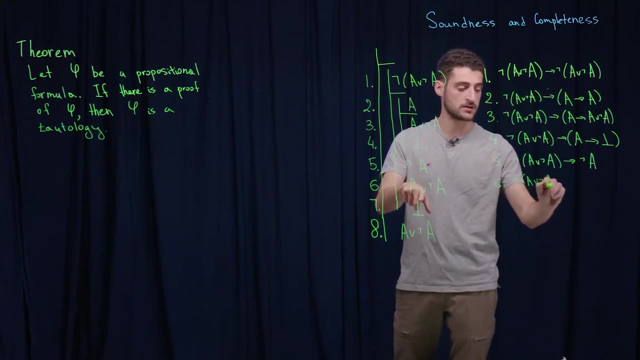 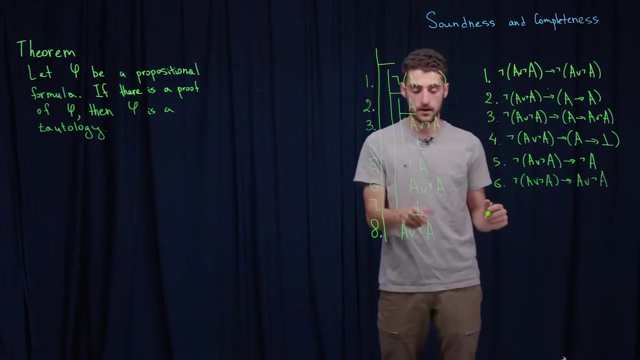 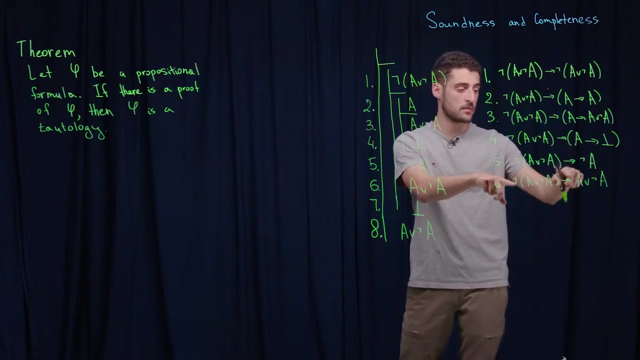 true. Now we have a sixth step and it's saying that, under the assumption that A or not A is not true, we can prove A or not A, And this is a tautology, because this is a tautology and we just replay the conclusion by A or this conclusion. 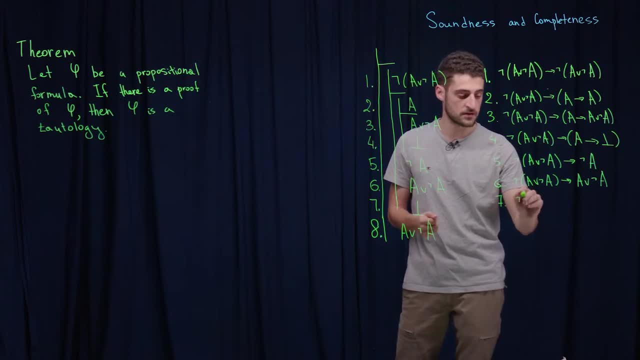 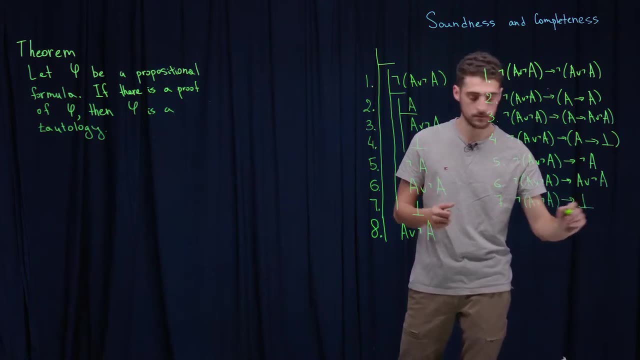 Finally, the seventh step is that, under the assumption that A or not A is false, we get a contradiction And this is a contradiction, This is a tautology, because this is a tautology, and we have assumption and the conclusion and they're opposites, so we get a contradiction together. Finally, the 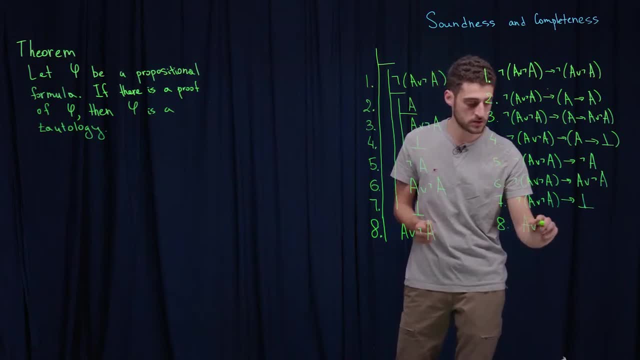 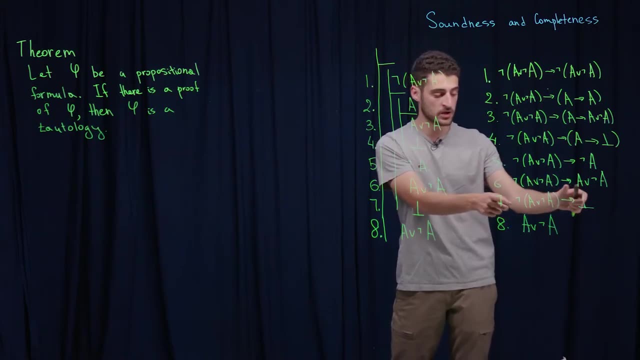 last step is A or not A, and this is a tautology, just because the seventh step said that if you have an assumption, you get a contradiction. So the assumption was wrong and, in other words, A or not A is a tautology And it finishes the 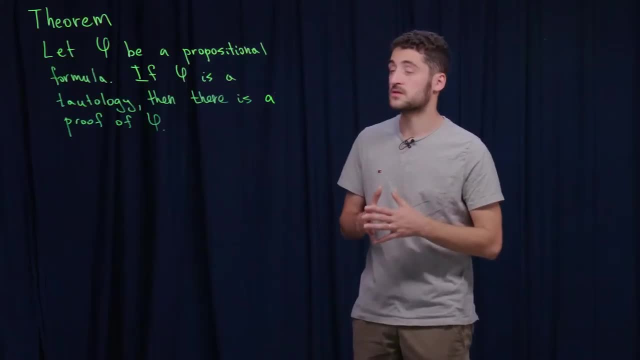 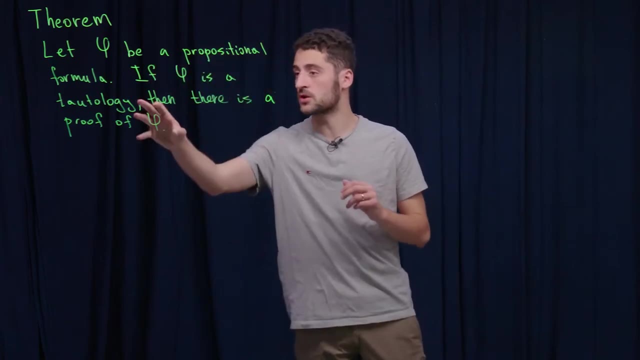 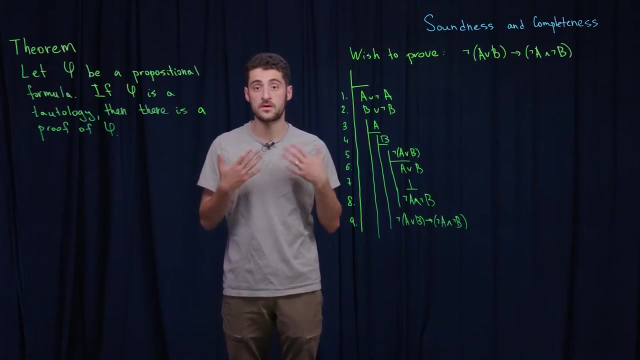 proof. The next property we're going to discuss is completeness, and formally it says like this: If you have a propositional formula and this formula is a tautology, then there is a proof of this formula. This theorem is actually even more involved than the previous one, so we 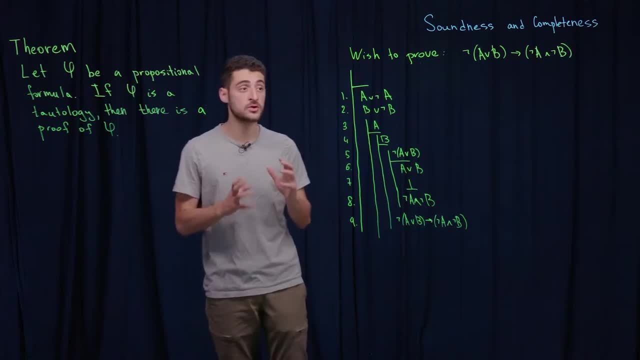 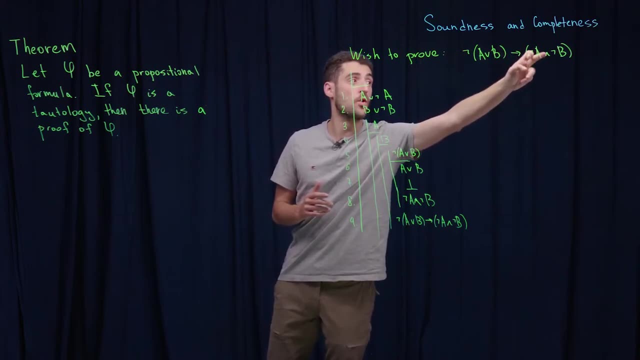 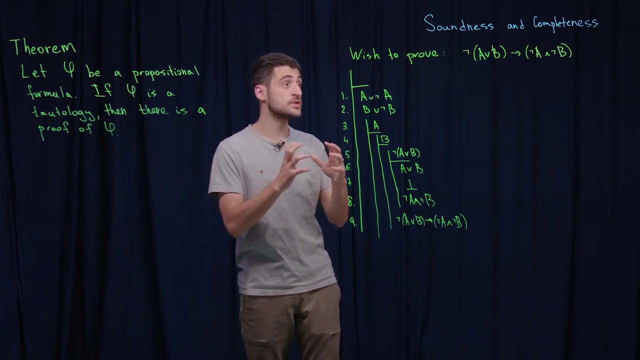 again illustrated within an example. Let's try to prove that negation of A or B implies not A and not B, In other words. so whether giving be or not B, it's a De Morgan's law. The idea of the proof is the following: We are going to 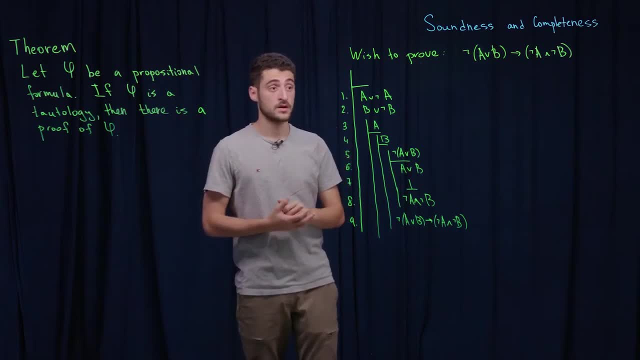 simulate the proof by truth table. In order to do this, on the first two steps we derive that A or not A and B or not B. Note that these are actual derivations. We need to make several steps in order to do this, but imagine that we already. 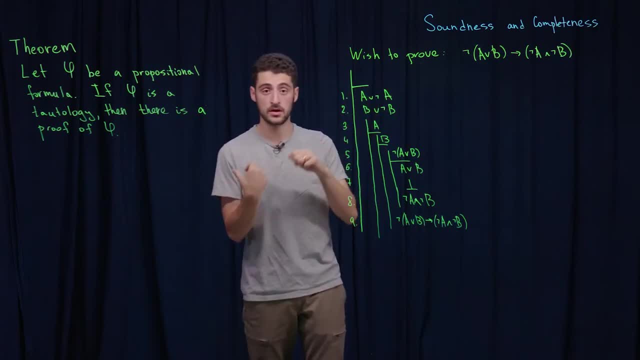 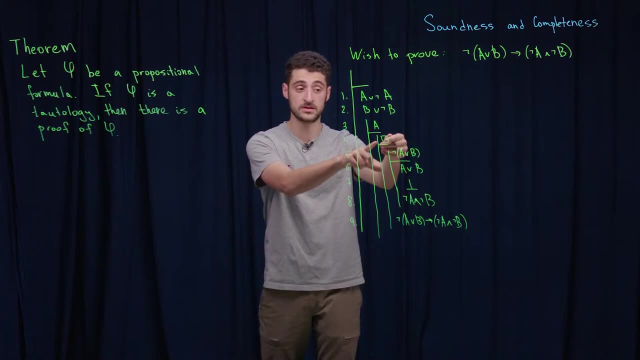 have them. The next step is to consider cases: if A is true or not A is true. Inside of both of these cases, you need to consider the cases if B is true or not B is true. Let's consider the first out of these four cases, when A is true. 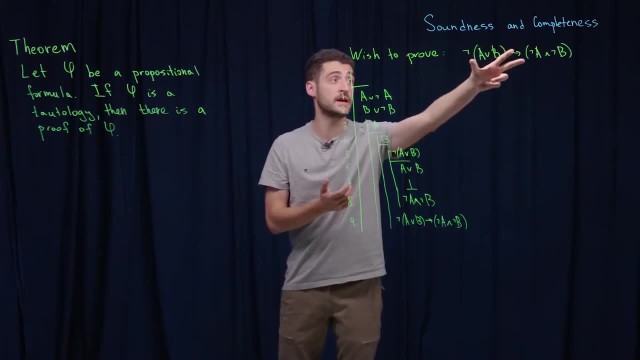 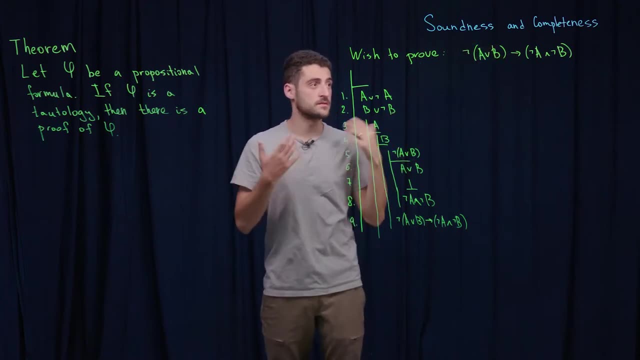 and B is true. We need to prove that in this case, this implication is true. In order to do this, let's assume that not A or B. After that, we may notice that this is actually false, under the assumption that A and B you. 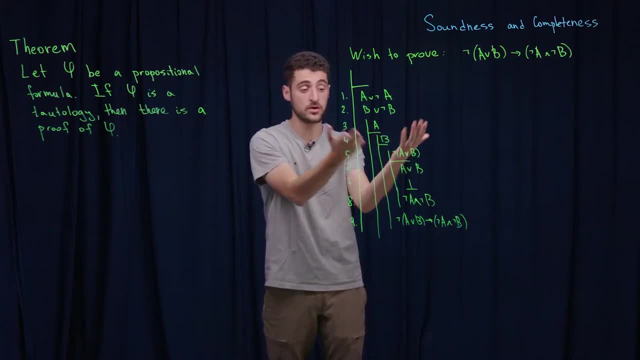 are true, because A or B in this case is true and negation is false. So we can derive the contradiction and after that we can derive this. So we notice that we have A and B. so we can derive A or B using the introduction of the junction. 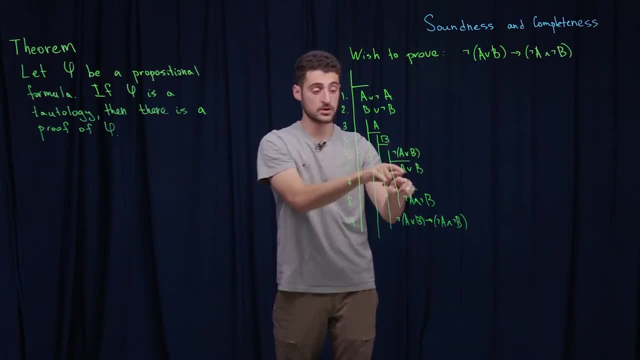 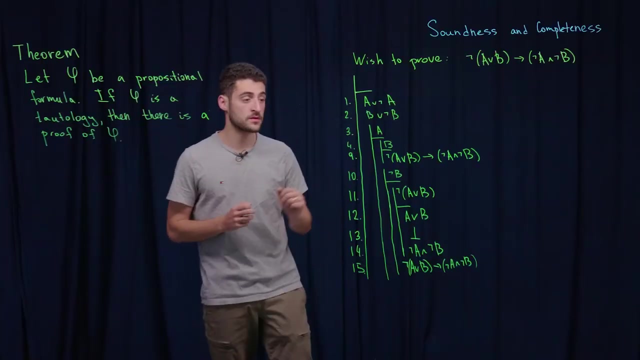 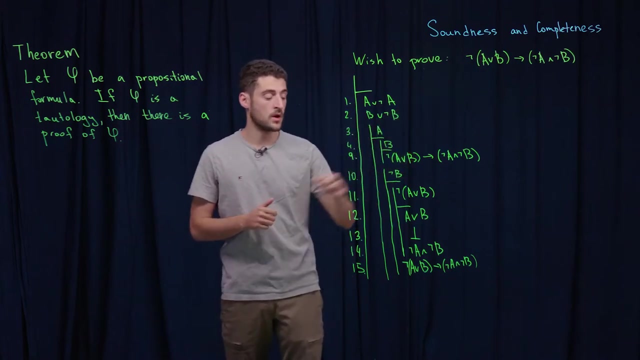 Note that it contradicts to the assumption. so we can derive a contradiction And from the contradiction we can derive everything, including not A and not B. And since with this assumption we can derive this, we can derive the implication. So we proved that if A and B assumed, we can derive this. Now let's consider the 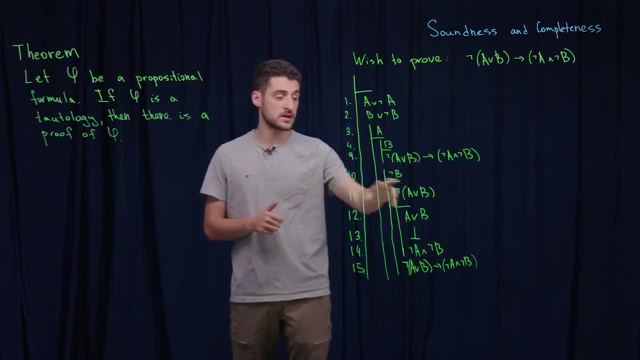 case when A is true and not B is true. In this case, again, we made an assumption that not A or B and we know A, so we can derive A or B And remember that since A is true, the assumption is false, so we need to get a contradiction. 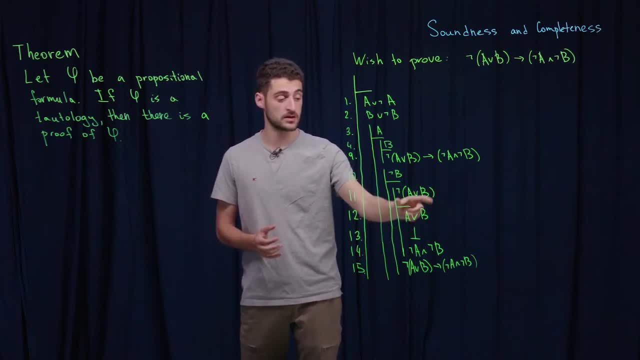 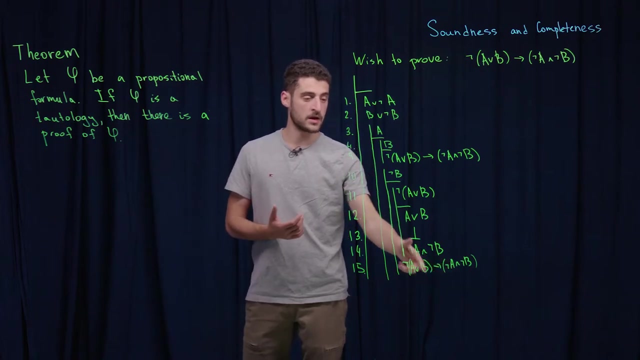 So, but A or B contradicts to the assumption. so we get a contradiction and we can derive everything, including the conjunction of not A and not B. In other words, we can prove the implication And in other words, in the if A is true, using B or not B. 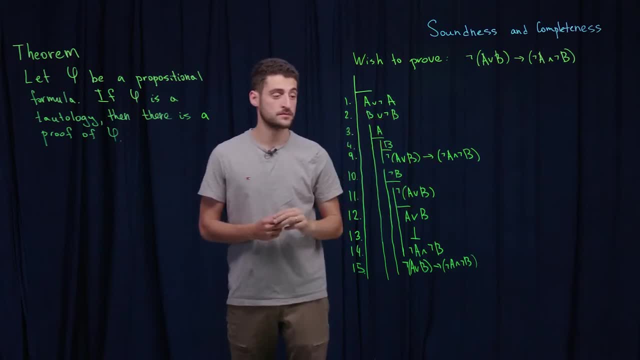 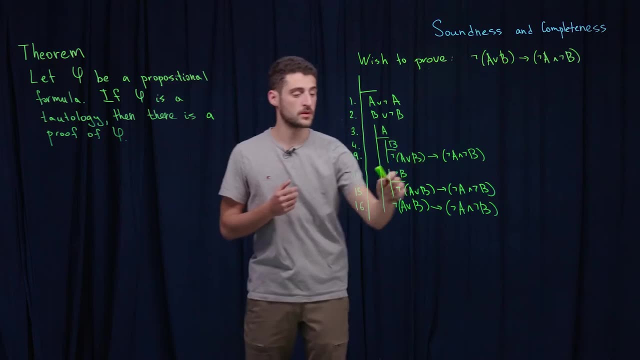 we can derive everything we want. So we prove that if A is assumed and B is is assumed, we can derive this. We also proved that if A assumed and not B is assumed, we also can derive this Using the fact that A or not A should be true. 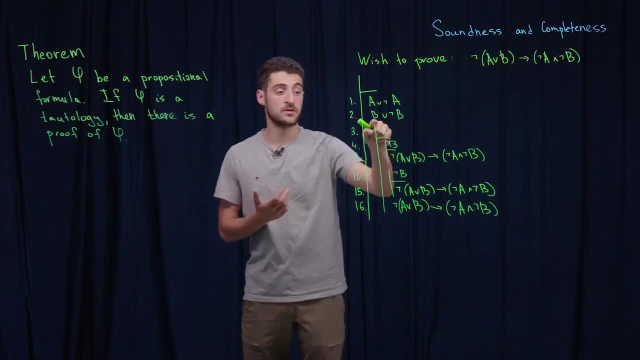 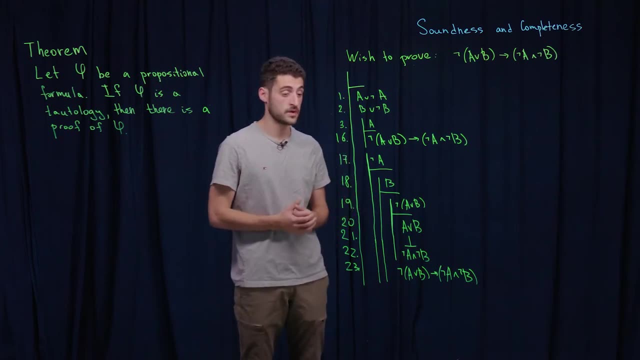 we can derive this under the assumption A: We consider the case when A is true. Now we need to consider the case when not A is true. And again we need to consider two cases for B and not B. First the case when B is true, So we know that, not A. 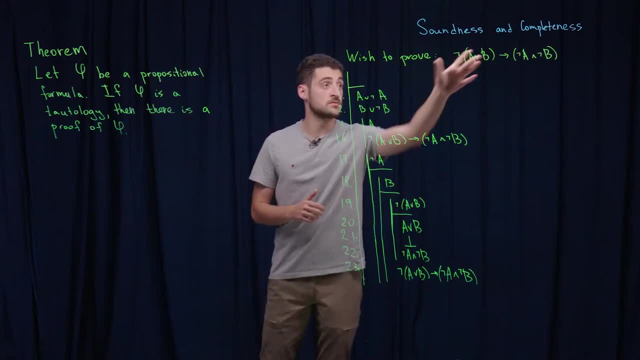 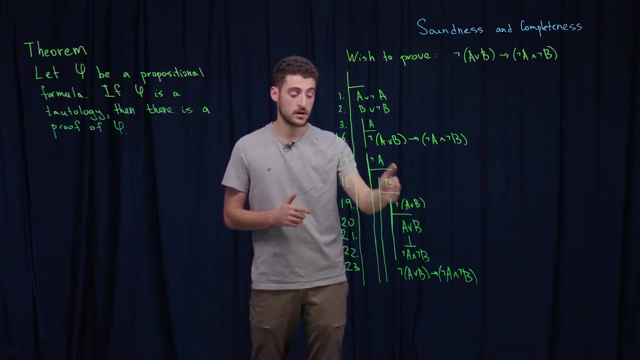 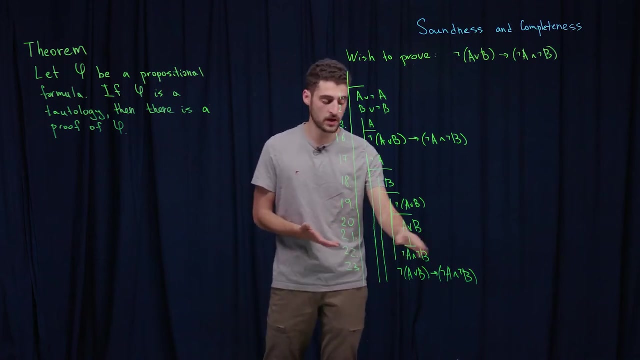 is true and B is true. Again, let's assume this. Note that B contradicts to this. because A or B is true, We can derive it from B using introduction over the disjunction And this together gives a contradiction. And we can derive everything from the contradiction, including not A and not B. 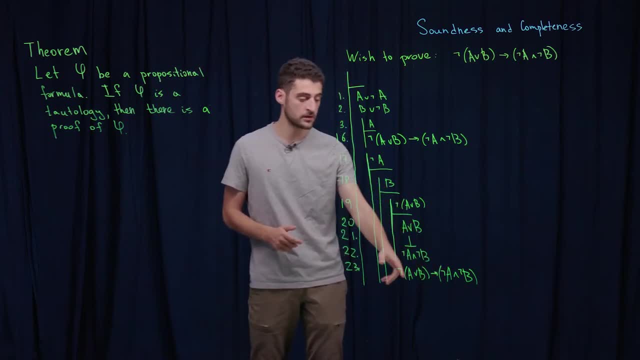 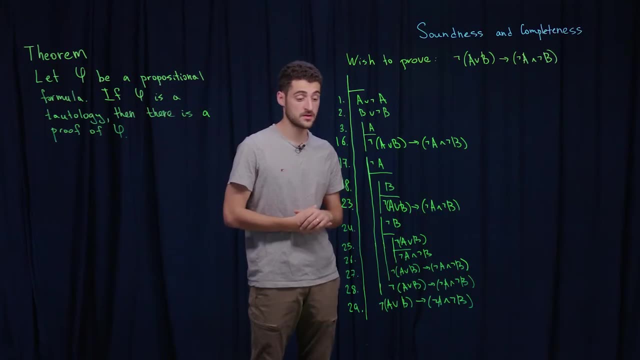 So, using introduction of the implication we can derive from this. this implication And the last case we need to consider is when not A is true and not B is true. Note that in this case we again need to assume this, And this time, not A and not B are not contradicting this.